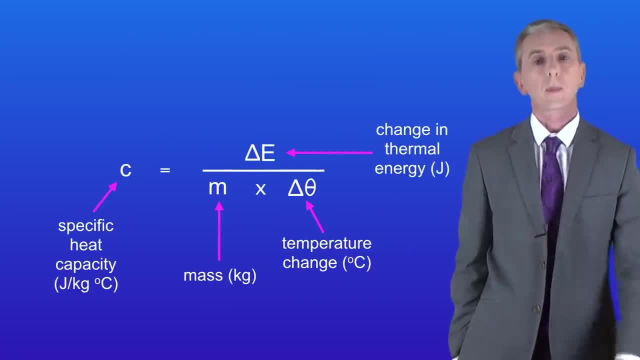 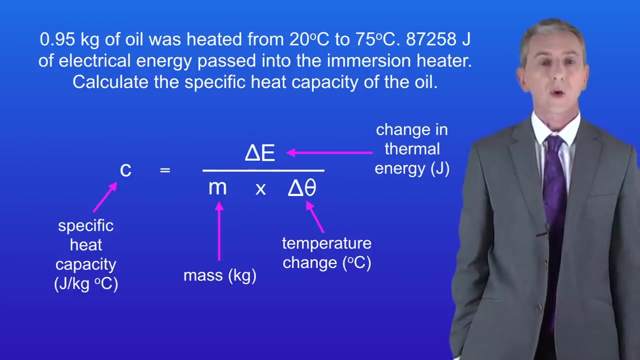 equation for specific heat capacity. and here it is. The specific heat capacity is a change in thermal energy divided by the mass multiplied by the temperature change. So here are the results of the experiment: 0.95 kilograms of oil was heated from 20 degrees Celsius to 75 degrees Celsius. 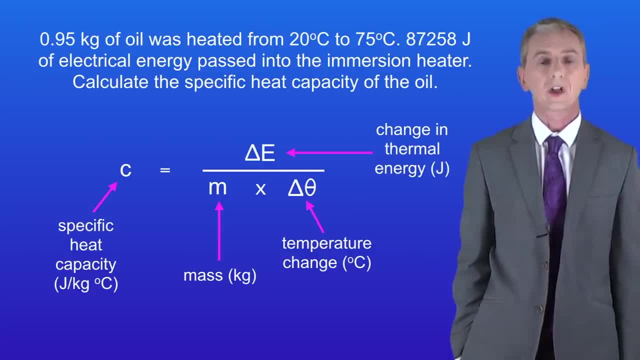 87,258 joules of electrical energy passed into the immersion heater. Calculate the specific capacity of the oil. So the change in thermal energy is 87,258 joules, The mass is 0.95 kilograms and the temperature change is 55 degrees Celsius. Putting these numbers into the equation gives us: 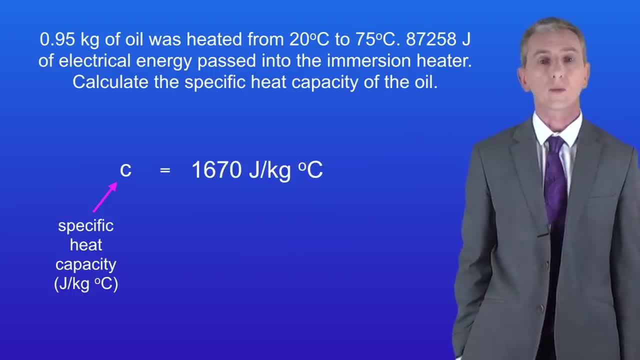 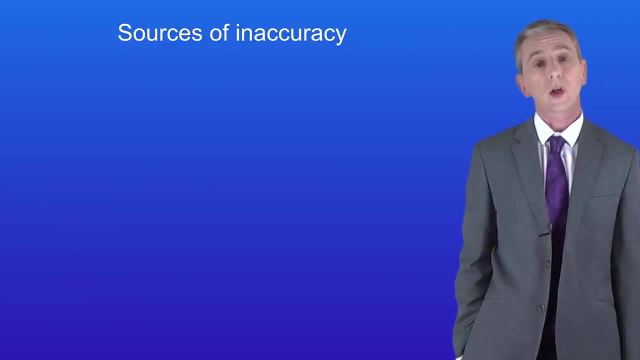 a specific heat capacity of 1,670 joules per kilogram per degree Celsius. Now the specific capacity that we've calculated may not be fully accurate, and there are a few reasons for this, So we're going to look at these now. The first problem is thermal energy passing out of the beaker and 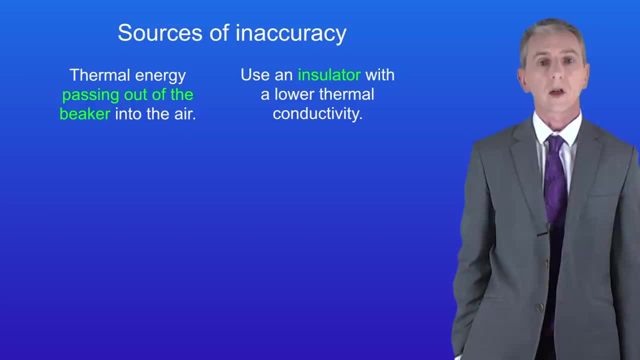 into the air. Now we can reduce this by using an insulator with a lower thermal conductivity and we'll be looking at the temperature change. So we'll be looking at the temperature change and we'll be looking at thermal conductivity in a later video. Secondly, not all of the thermal 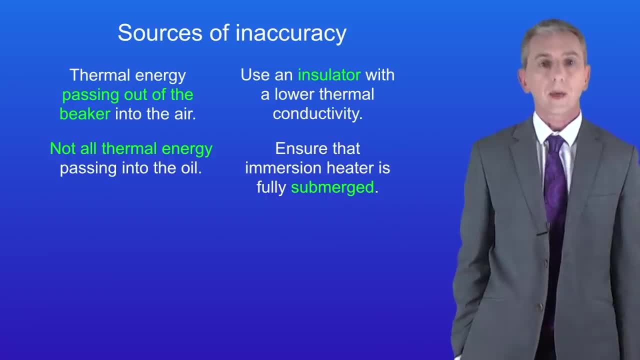 energy from the immersion heater passes into the oil, and we can overcome that by ensuring that the immersion heater is fully submerged. The next problem is incorrectly reading the thermometer, and to prevent that we can use an electronic temperature probe. Finally, thermal energy may not be spread through the oil, and to reduce that error, 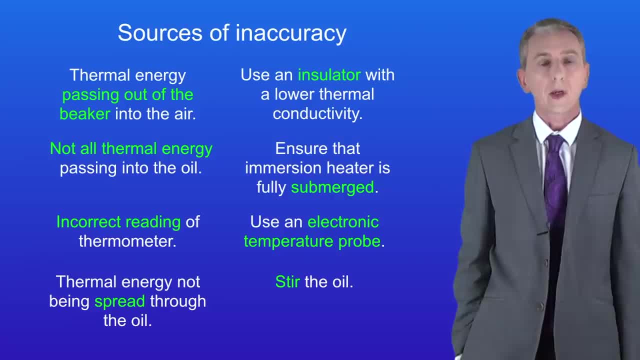 we can stir the oil Now. I should point out that there will be other minor sources of inaccuracies, but these are the main ones. You'll find plenty of questions on this required practical and all the others in my revision workbook and you can get that by clicking. 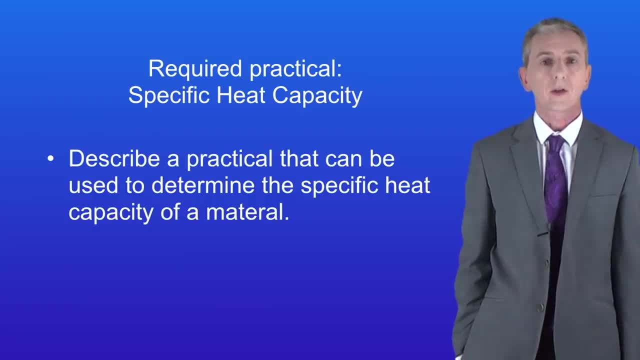 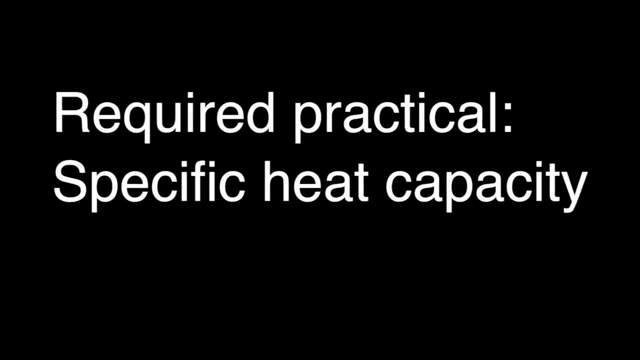 on the link above. Okay, so hopefully now you should be able to discover a practical that can be used to determine the specific heat capacity of a material.